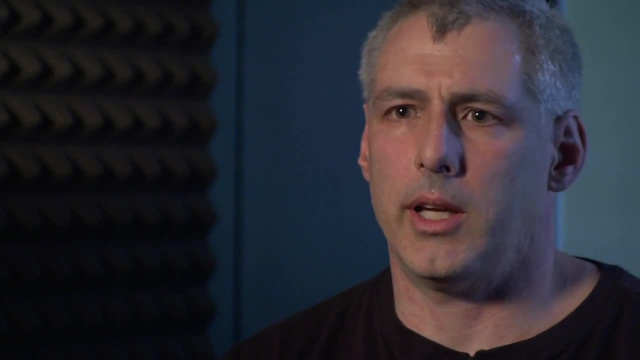 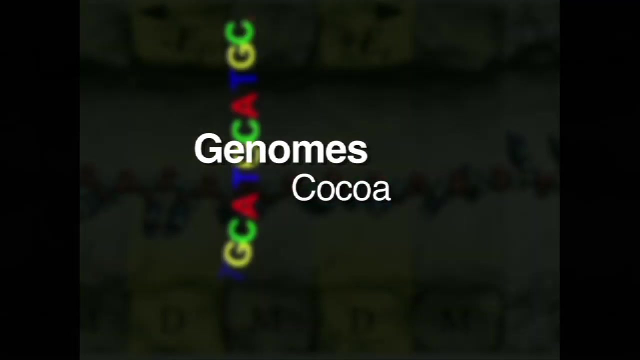 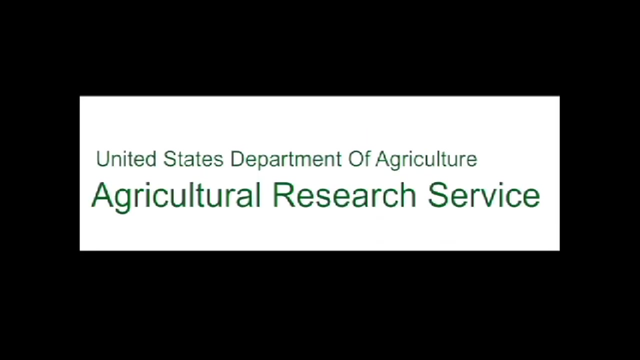 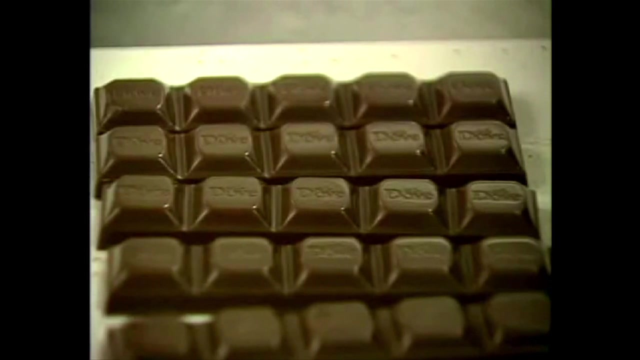 chlamysomal cells. It takes almost anything to produce bioexperience, to create an algorithm and to 69% much cancel something. This work takes days and hours. it takes prec, Pause, 3 Time, 5, 3, 7, 1, which is cocoa, which is the main ingredient that goes into chocolate that we all enjoy. 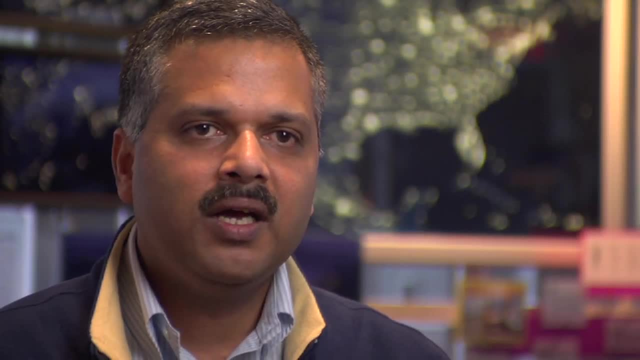 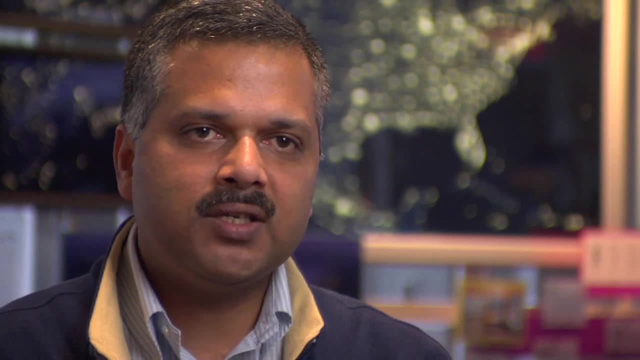 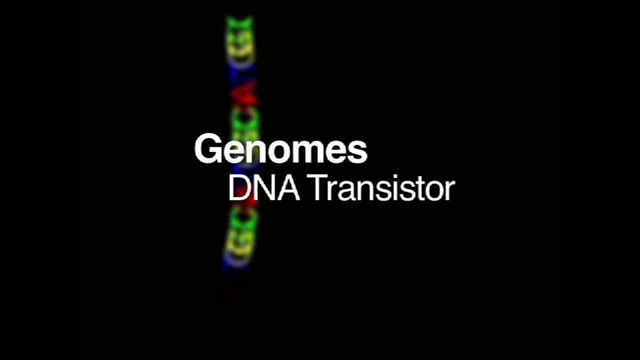 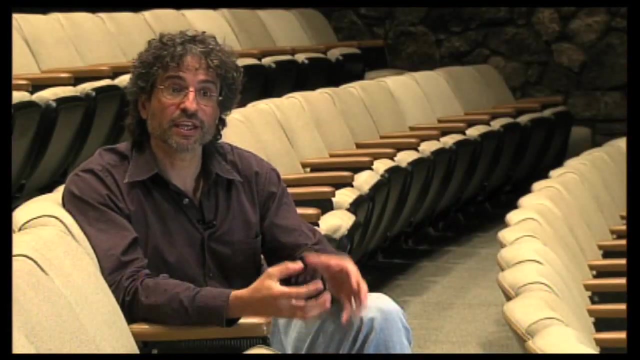 The goal of looking at the genome of cacao is to understand what variations correlate to produce desirable traits such as tolerance to pests and increased yields in the face of drought. What we are trying to do with the DNA transistor is to sequence DNA. We want to control the passage of DNA through a pore. 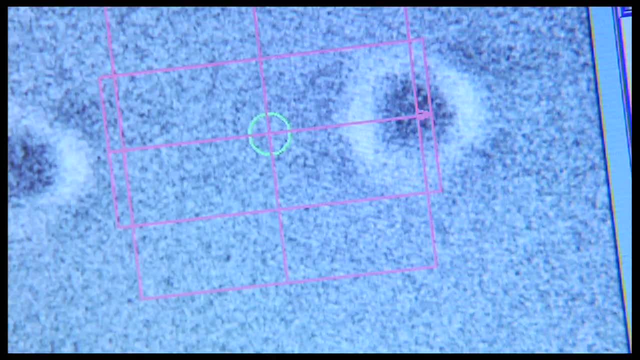 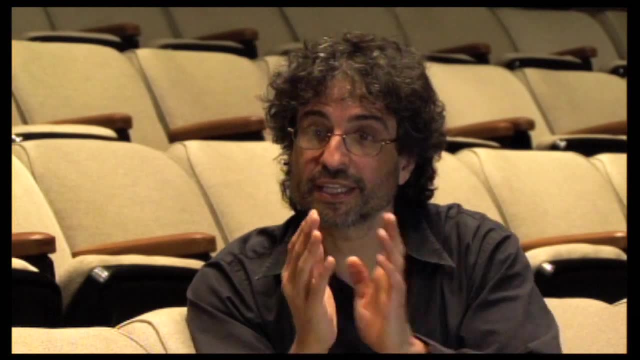 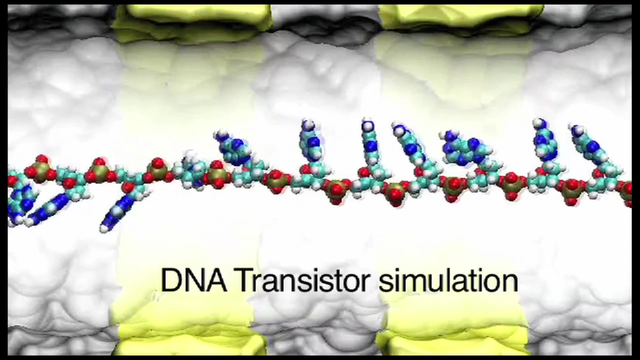 This device that is formed by a pore and a few electrodes allows us to make a DNA go through this little pore and be trapped by the electric field created in these electrodes. As much as trapped, we also can get rid of this electric field and the DNA will traverse. 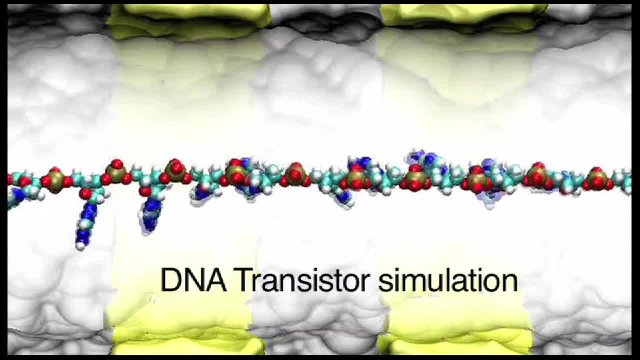 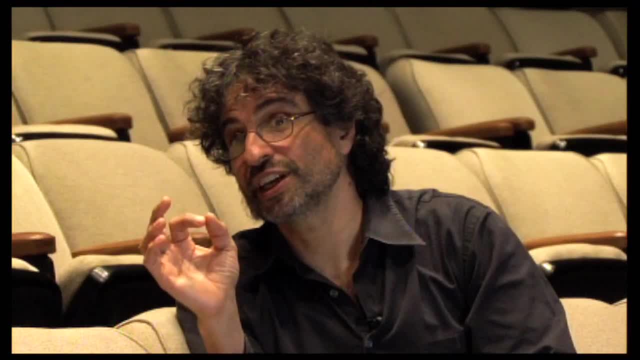 through the pore a little bit and we trap it again. And each time we trap the DNA we can do something with it. For example, interrogate each base And ask: are you a C, a G, an A or a T? 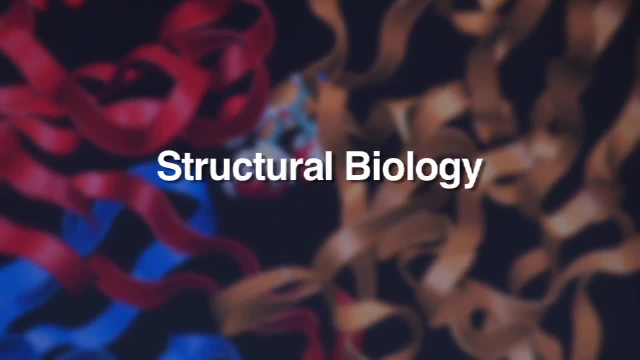 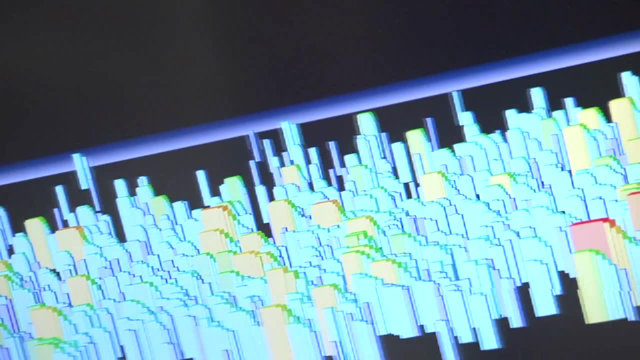 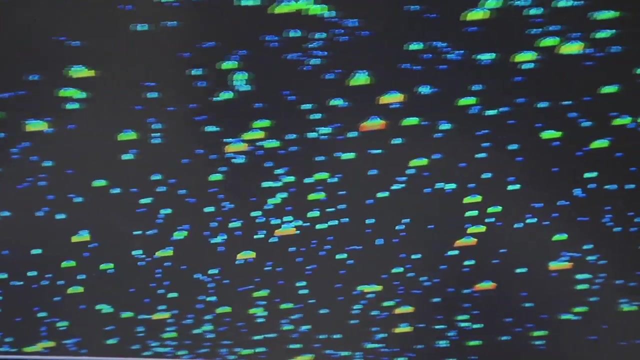 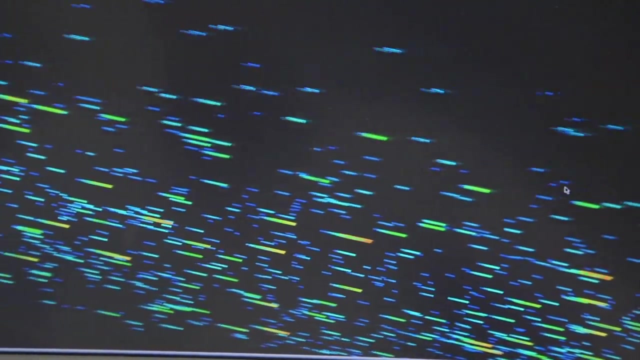 And that will allow us to sequence the DNA Projects in structural biology include simulating structures of proteins and protein-protein complexes. So these are three-dimensional structures that we simulate using supercomputing technology such as Blue Gene, And the goals of such study is to understand how protein structures behave and what variation. 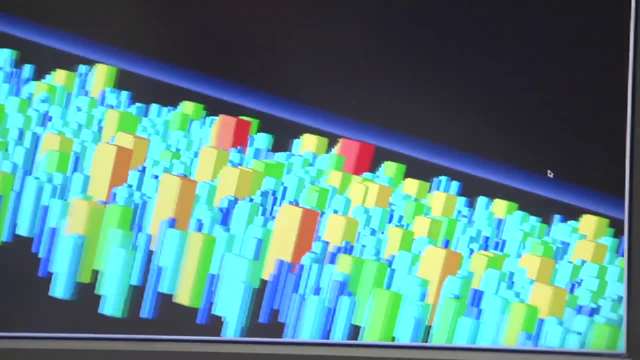 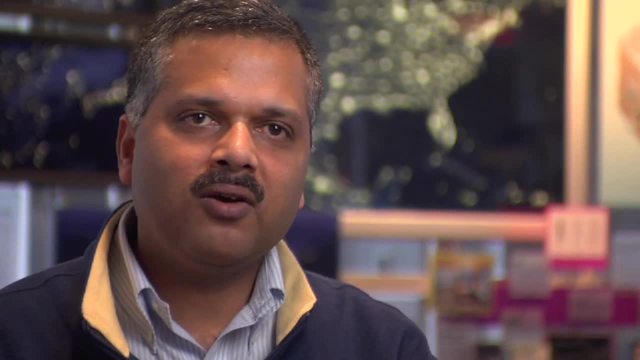 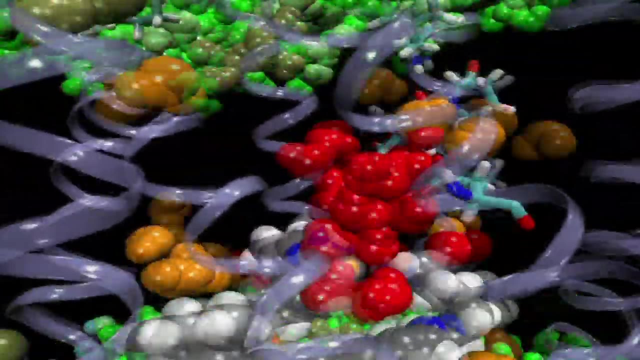 in the protein structure results in what kind of biological change. We are engaged in two such projects, The first of which I want to describe is work we are doing on the protein called rhodopsin. We study the protein rhodopsin because it is the protein in the retina of our eyes. 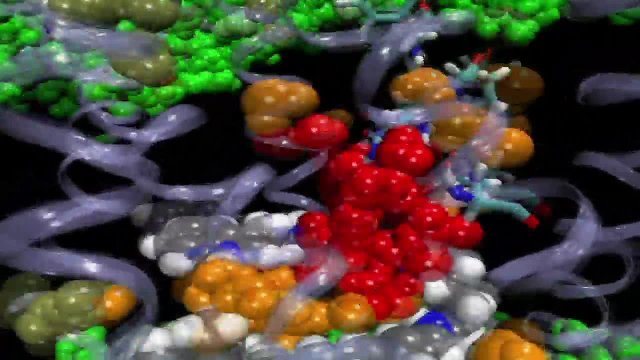 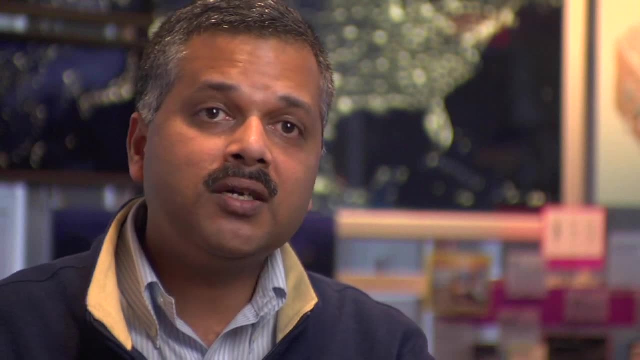 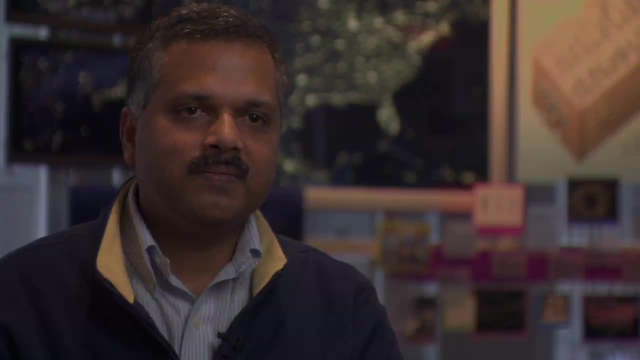 Its job is to receive a photon of light and transduce that into a chemical signal Using protein simulations. we ask the question: how does rhodopsin behave? How does rhodopsin do this job? The second area of research is protein simulations in influenza. 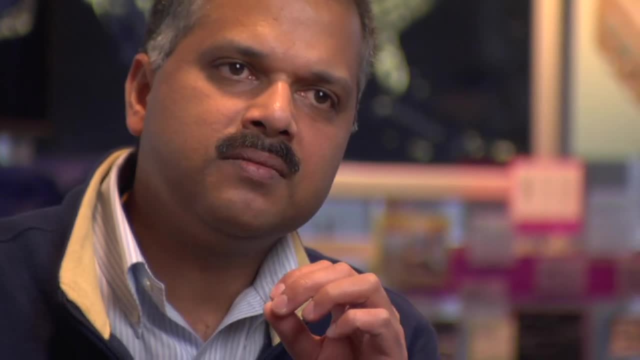 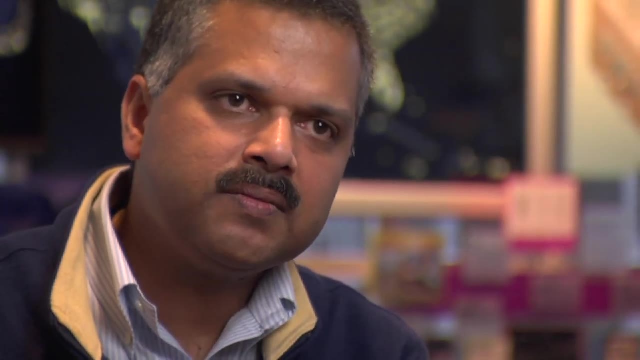 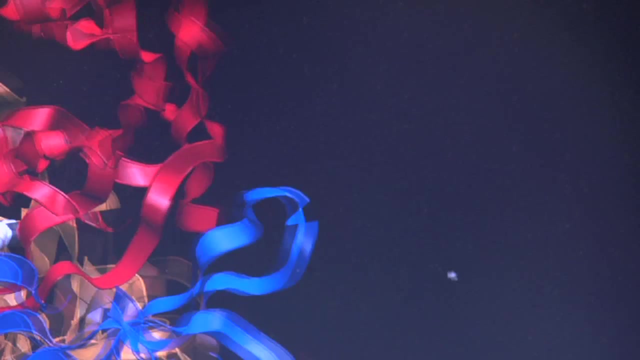 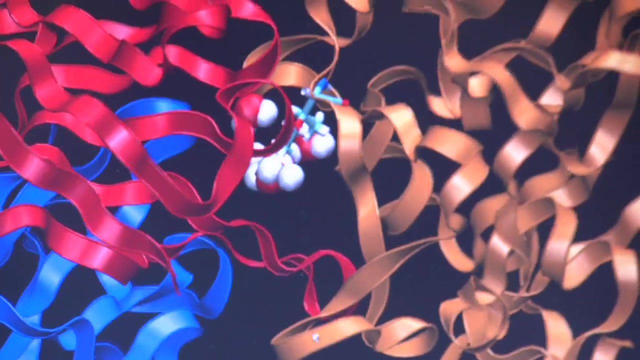 Influenza virus succeeds in making infections by constantly accumulating new mutations. Using sophisticated protein simulations, our goal is to predict what mutations are likely to occur on influenza virus, And then what new antibodies or vaccines could be developed to recognize these. as yet, 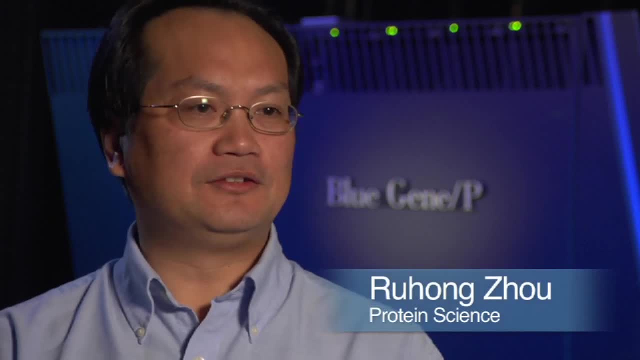 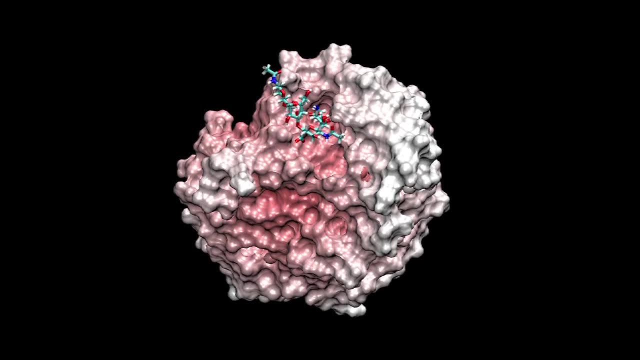 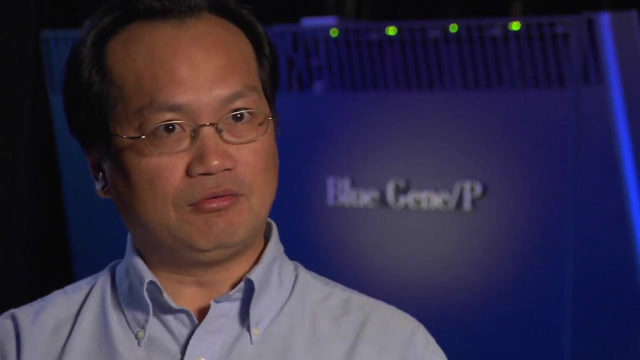 unseen mutations. There are several questions we try to address, For example, why avian flu H5N1 only binds to avians, not to humans, And why some mutations will cause the escape of antibody neutralization. And a third type of problem. we are working with University of Rochester at this moment. 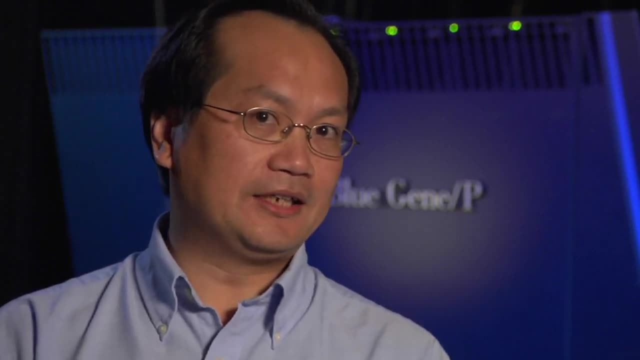 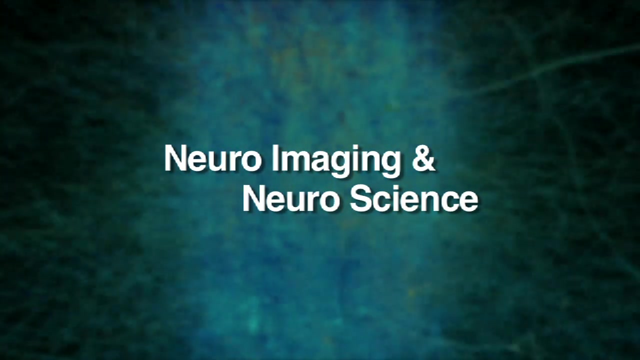 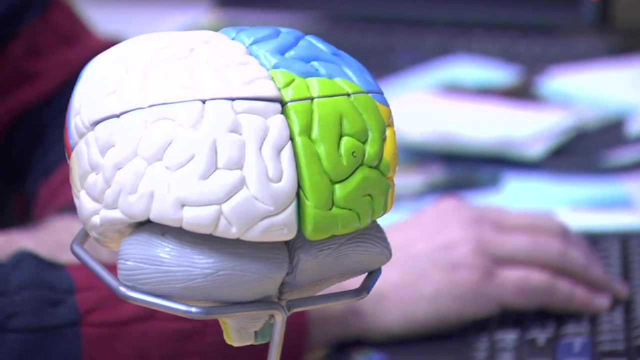 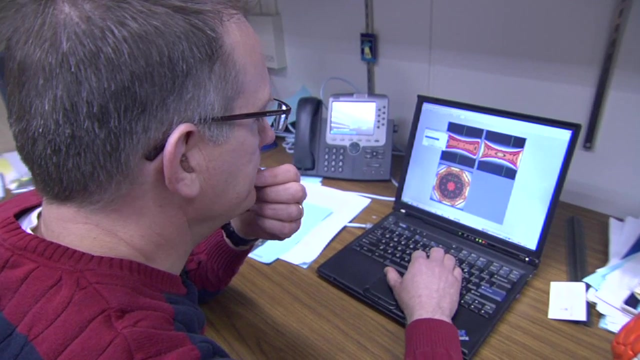 was why some of the T cell response will attack some of the virus peptides, but not the others. We collaborate with neuroscientists around the world to build models of how pieces of the brain assemble and behave to give rise to the complex functionality that we associate. 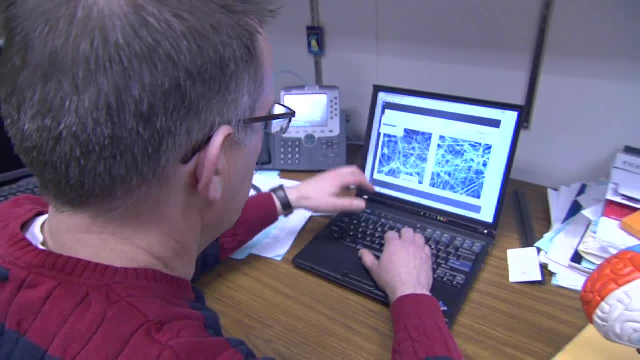 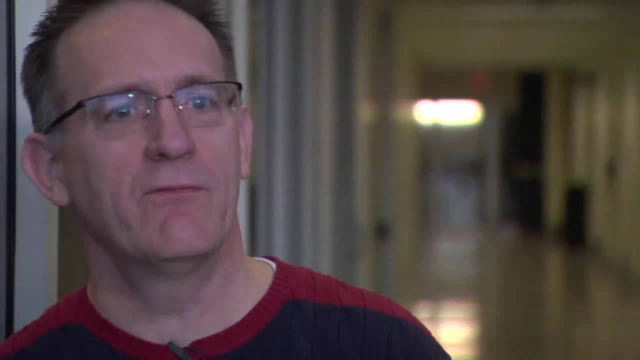 with the behavior. For example, we are studying the emotion. We are studying the emotion control system in the brain that gives rise to things like fear and phobia. One specific research project we have is working with a group in France called NeuroSpin. 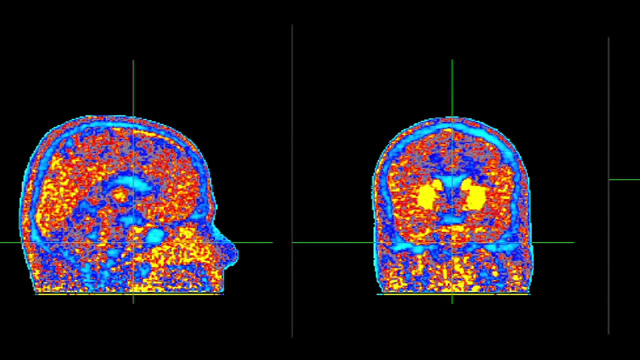 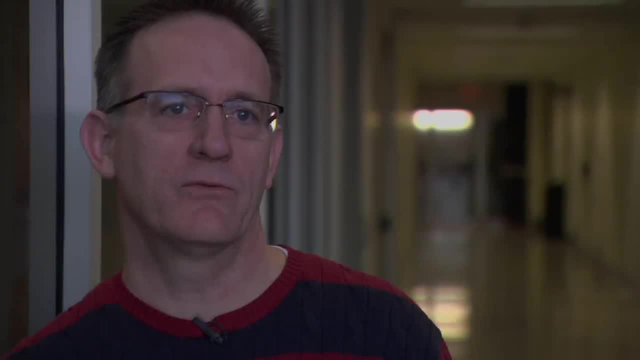 And what we are trying to do is to develop techniques that can distinguish between schizophrenic patients and normal patients. What we are trying to do is to understand or characterize the functional relationships the different areas of the brain have relative to each other. What is proteomics? 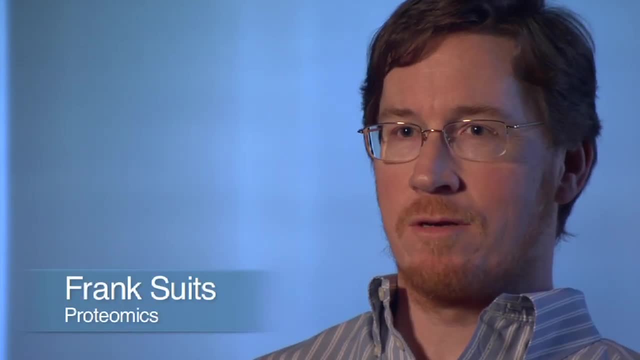 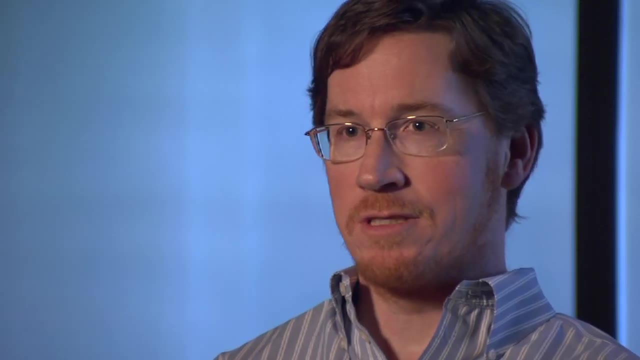 Proteomics involves actually studying the function of the brain, Studying the proteins as they appear in the body, including small modifications to them that might happen, related to disease. The hard part is actually understanding that data and finding the patterns that might have the biological signal you're after. 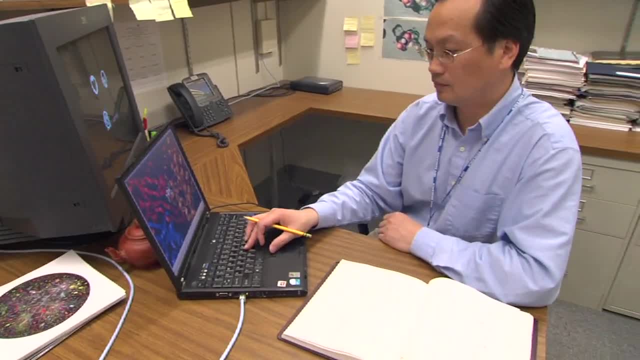 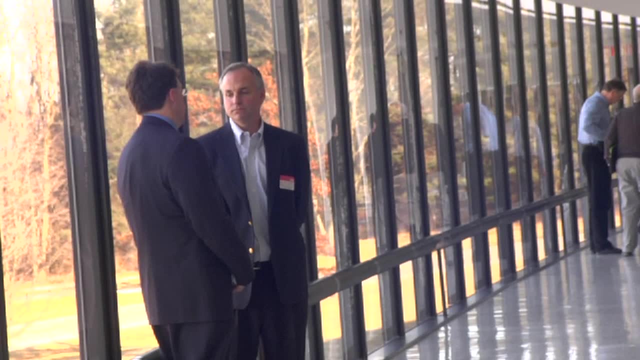 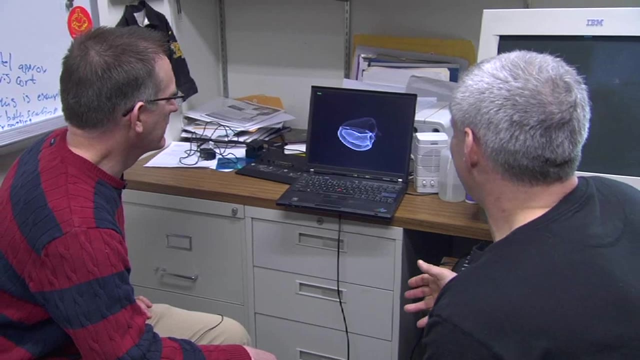 Our strategy of working in this space of computational biology is to collaborate with researchers and institutions around the world. Take our expertise at the intersection of information technology and biology, combine that with bench biologists, Join experimentalists and leading scientists in this field and together make progress.